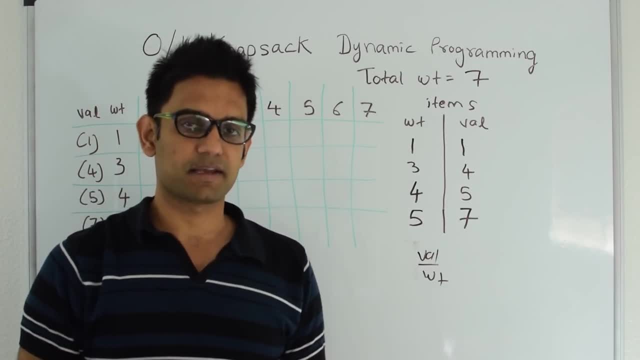 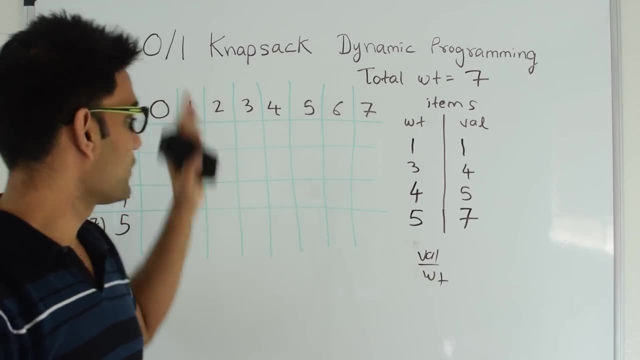 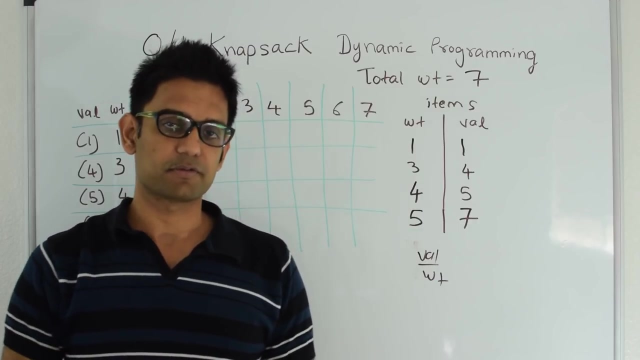 picking the items and then, if the last item cannot be picked, totally split it up and pick whatever ratio you can. So, but here we are doing 0-1 knapsack problem. It means that we cannot split the item. So how do we do it? Yes, we will use dynamic programming to solve this. 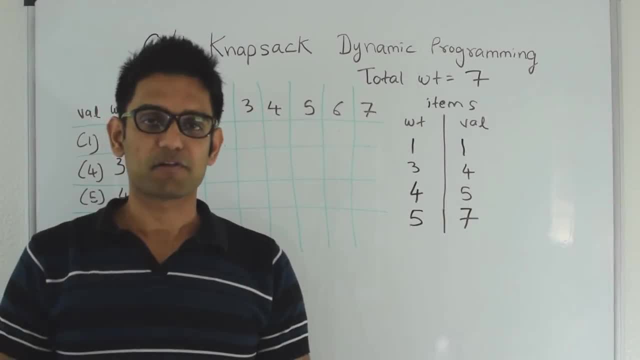 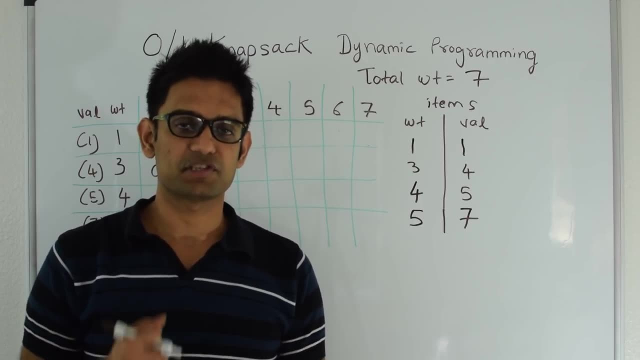 question. In the next section let's see how. So how do we solve this problem? So the question is very simple: Whenever a new item comes in, you have to decide if you have to pick this item or not, and you have to find which gives you the maximum value. If you pick the item, the 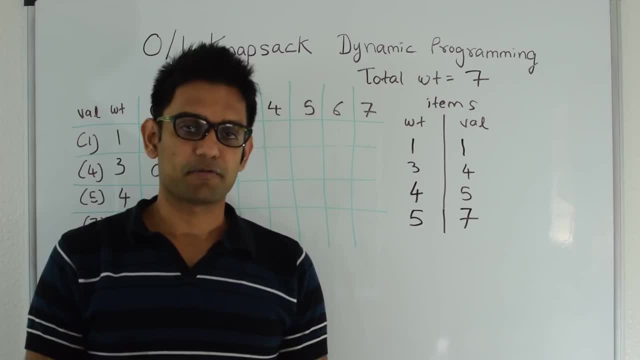 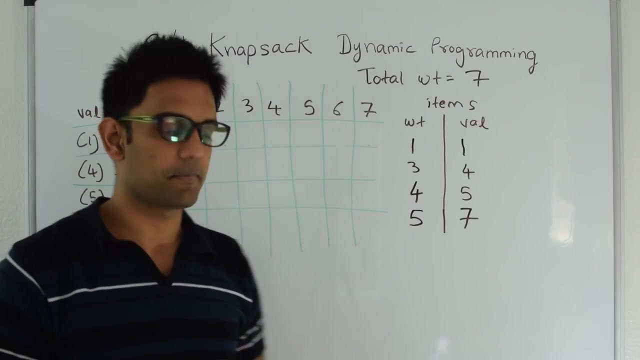 maximum value will be the value of the item plus whatever we can get by subtracting this value from the total weight and excluding this item, or the best you can do without including this item altogether. Let's try to understand on with this example. So here I have a two-dimensional 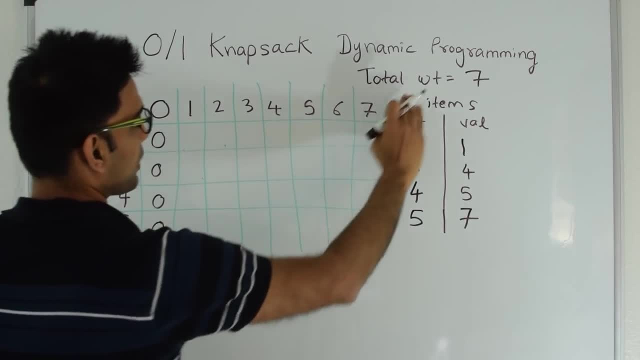 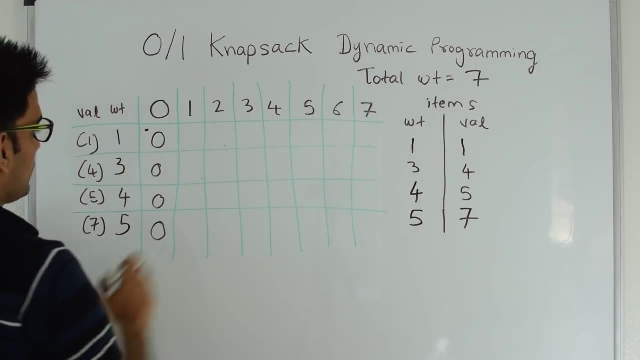 matrix, and this is my total. number of columns is same as the total weight plus 1, and my number of rows is same as the total items. So our first column is 0.. It means that if the total weight is 0,, no matter what items I have, my maximum value I can get is 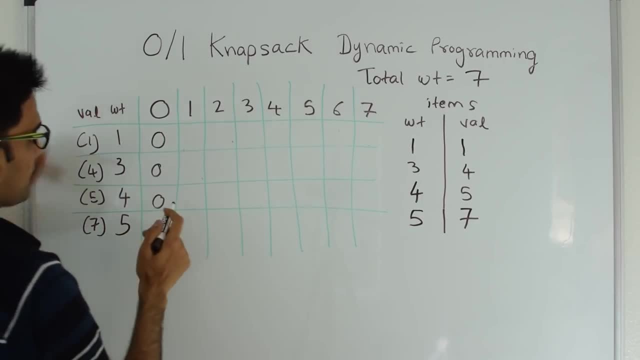 always 0. So this is why this all is 0.. So let's start from here. So if my total weight was 1 and if I just had one item 1, the best I can do is 1.. So this is the weight of the item. 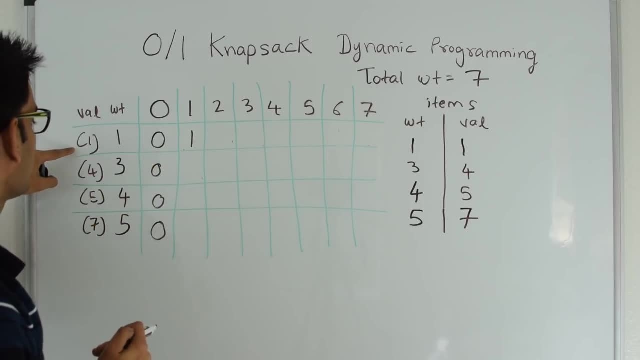 The total weight is 1.. So the maximum value I can get is just 1.. If my total weight is 2,, if I just had one item of weight 1 and whose value is 1,, the best I can do is 1.. 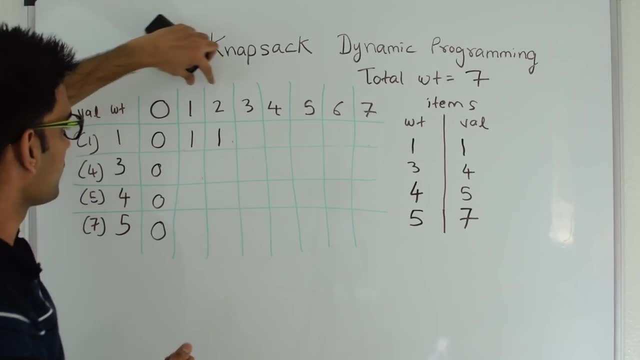 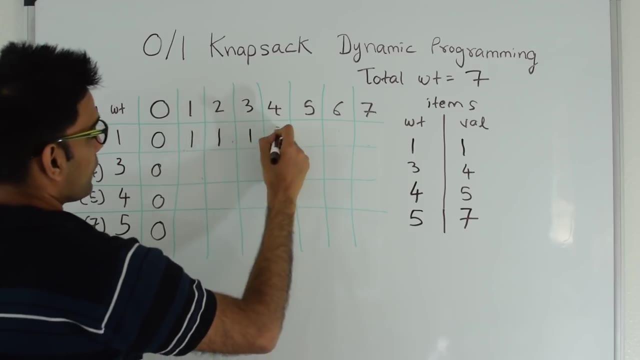 Remember, we just have one quantity of each items. So, even though the total weight is 2,, if I just have item 1, the best I can do is value 1.. Similarly, 1, 1, 1, 1, 1.. So if the total weight is 7, if the only item I have is 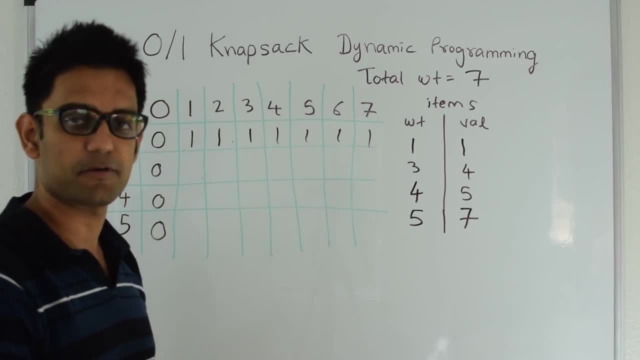 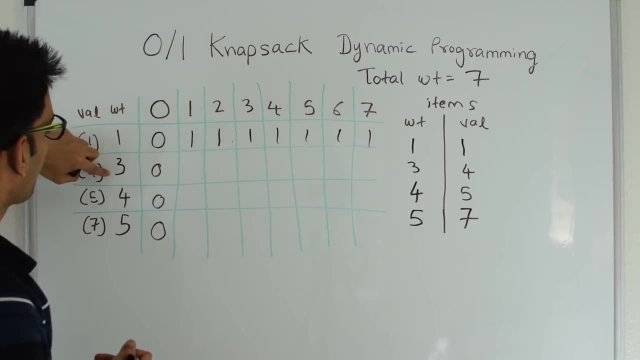 weight 1, and whose value is 1,, the best I can do is 1, because we have one quantity of each item. So next let's introduce 3.. So if the total weight is 1 and if the weight of the item is 3, 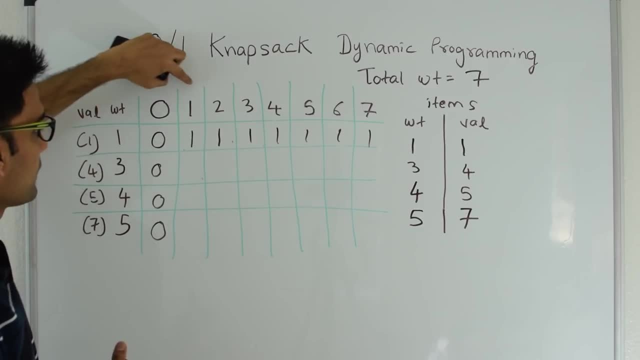 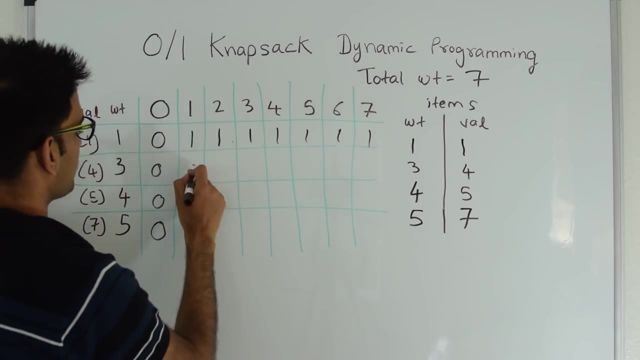 which is greater than the 1, so 3 can never be in the can never be selected. So what we do is: what is the best we can do without selecting 3?? So basically this number, So that's 1.. Again, 2.. Since 2 is less than 3, 3 can. 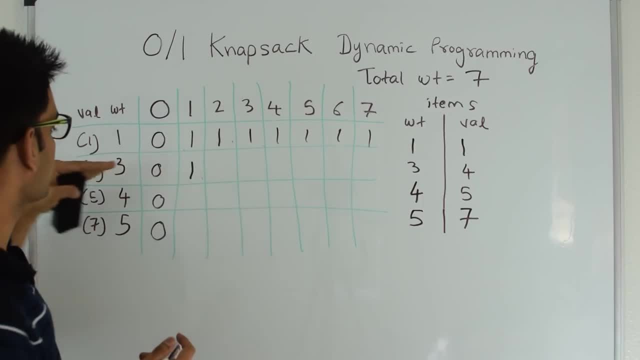 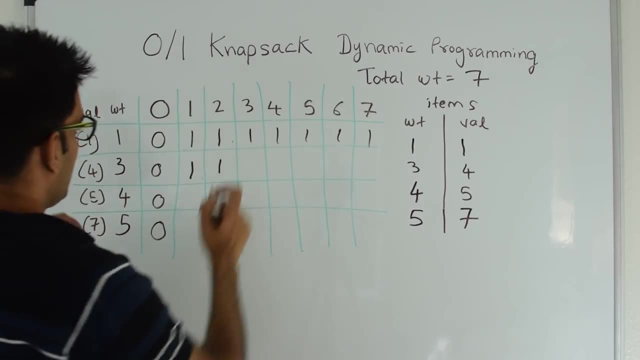 never be selected, since the total weight is less than 3.. So what is the best we can do is without 3,, what is the best we can do, which is this number, So that's 1, not 3.. So, since 3 is less than or equal to 3, we have two. 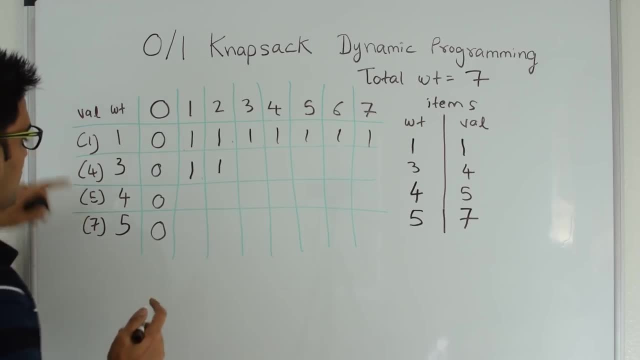 choices. Do we select 3 or do we not select 3?? If we select this item, so we have to check what is the best you can do by selecting this item. If we did select this item, this gives me a value 4 plus, whatever weight is. 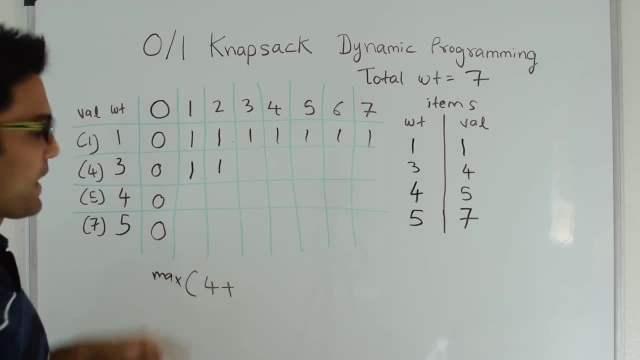 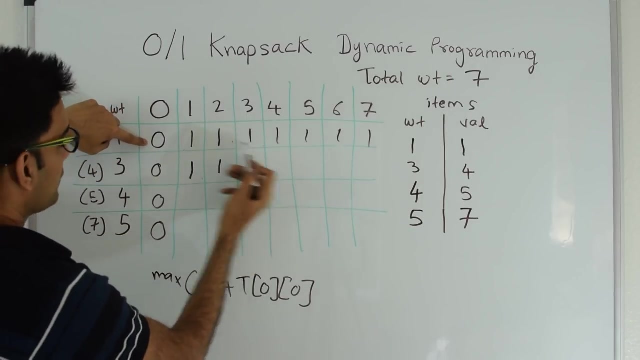 remaining after we select this weight. So 3 minus 3.. So that's 0. So t of 0, and then, and then we go to the top column, So that also 0. So we reach this point, So we go up, We go three steps. We reach this point Three steps, because the weight of 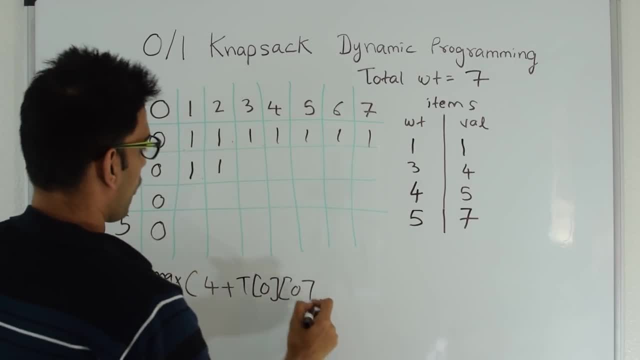 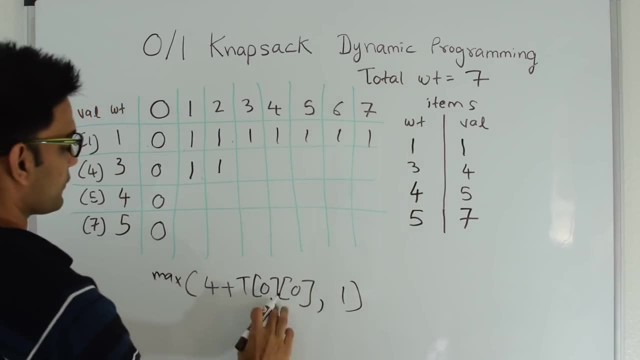 this item is 3.. So t of 0, 0 is 0. Or what is the best value we can do without selecting this item altogether, and that's 1.. So this value is 4 and this value is 1. So max of this is 4.. 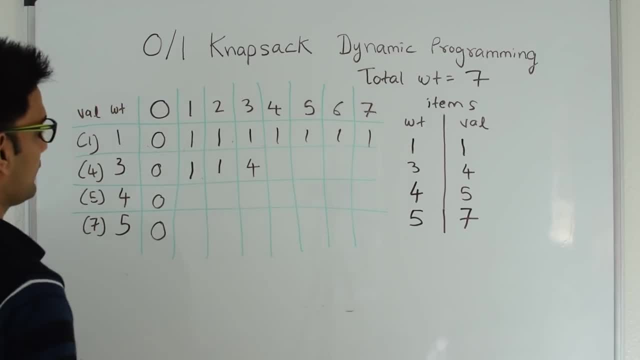 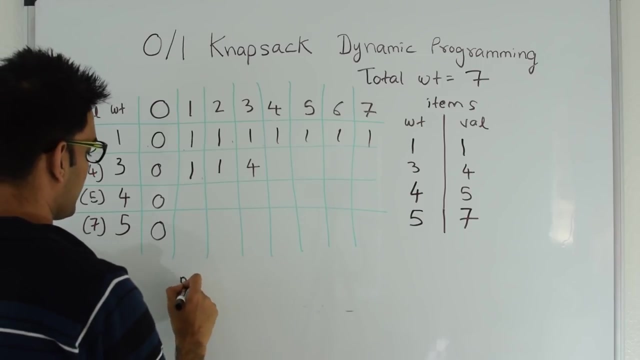 Alright, So the total weight is 4 and the item weight is 3.. So, again, the best I can do is without selecting 3, the best I'm getting is 1.. If I do select 3, the best I can get is max of. by selecting 3, I get a value of 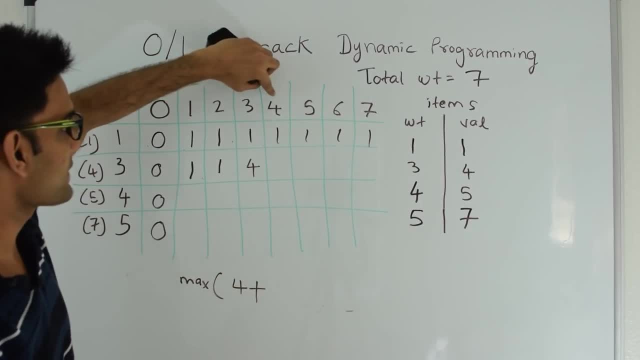 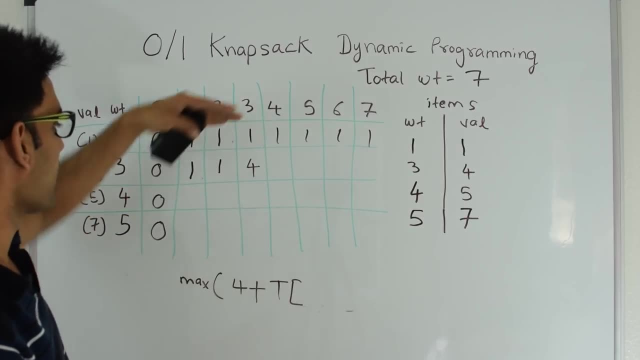 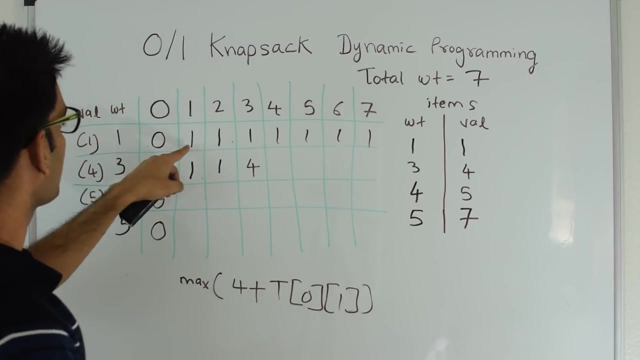 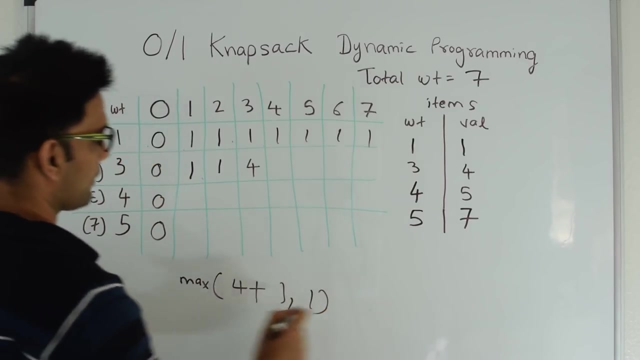 4 plus I subtract 3 from the 4. So that's 1.. And then I go one row up, which is 0 and 1.. So this value 0 and 1 is 1.. So 4 plus 1 is 5.. So max of 4 plus 1 is 5, or this value 1. So. 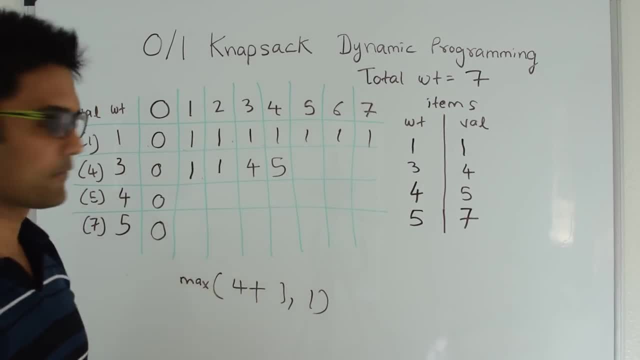 that's 5.. Again, where did this 1 come from? Since we selected this item, this I can use as a value of 4.. So what is the weight we are left with? The weight we are left with is 1, because 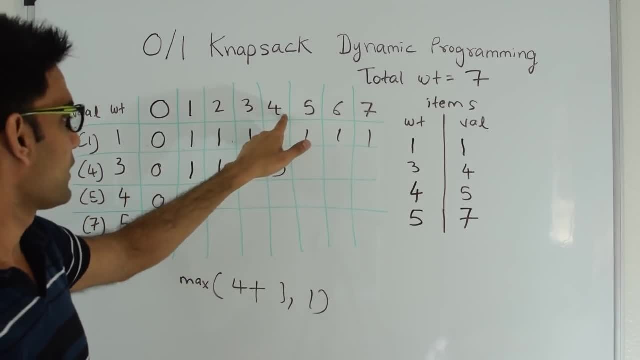 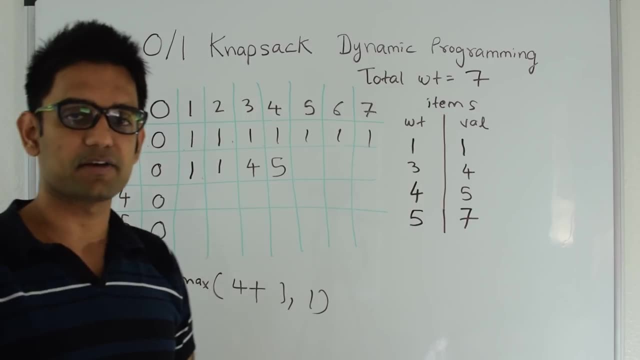 this guy is going to take 3 weight and our total weight is 4.. So we are left with the weight of 1, and then we checked what is the best we can do if we had just weight 1 and we did not include item 3.. So that's this guy here which is 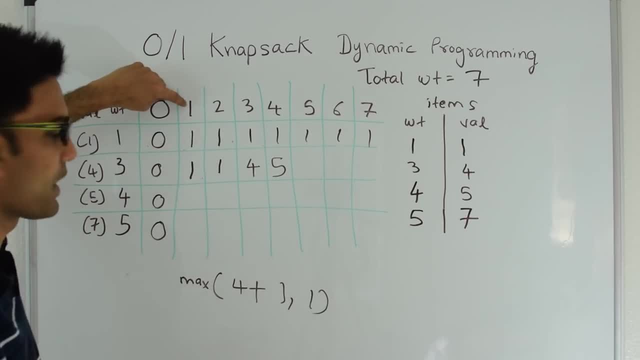 why we came to this point and the best we can do if we had a weight 1, total weight 1 and just item 1 is 1.. So that's how we get 4 plus 1,5, and the best we can do without including 3 is 1, so we get. 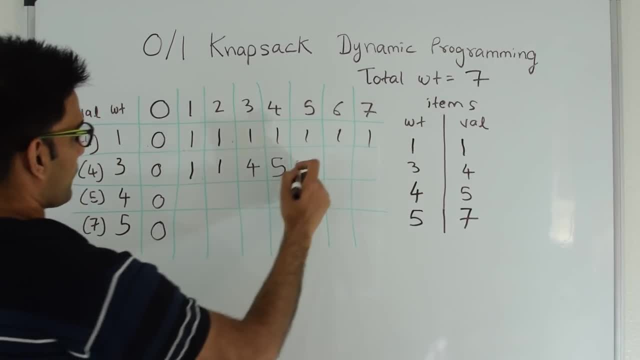 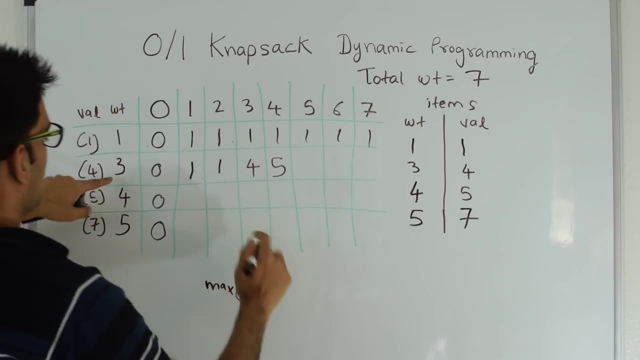 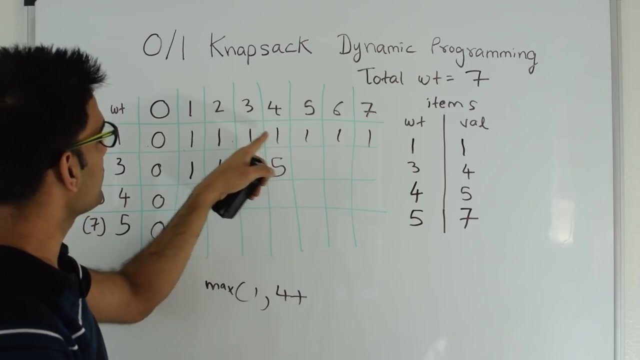 the max of that. so that's 5.. Alright, so 5 here. So again we are checking max of either 1 or weight of value of this guy, so that is 4 plus we go up and three steps back: 1,1,2,3, and. 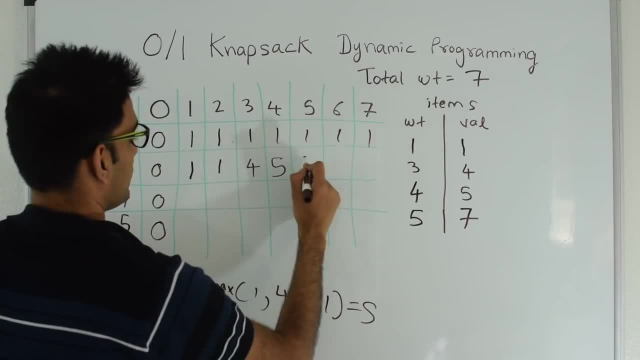 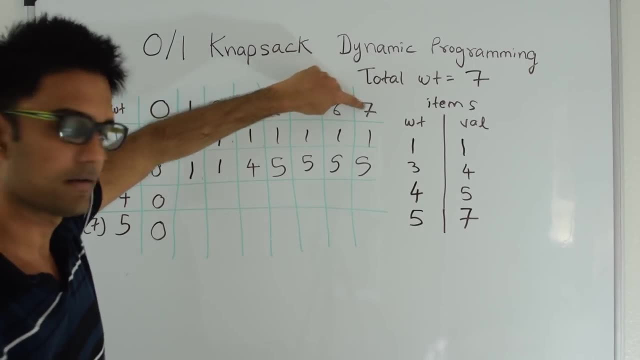 reach this point. So this guy. so that is 5.. So this value will be 5.. So it will be 5 all the way till the end. So if I had a weight, total weight 7- and if I had two items, 1 and 3, the best I can do, 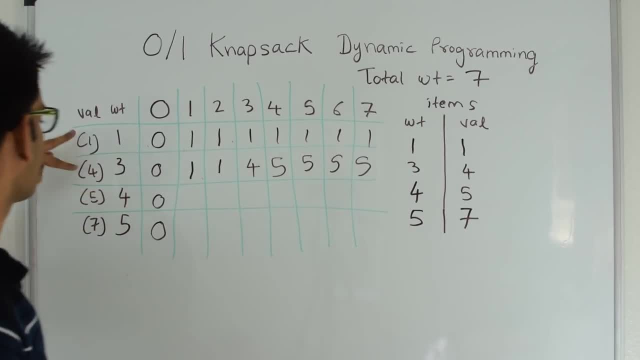 is. the maximum value I can get is 5, which is pretty much selecting both the items. Let's include 4.. So since 4 is less is greater than 1, this item cannot be picked if the total weight is 1.. 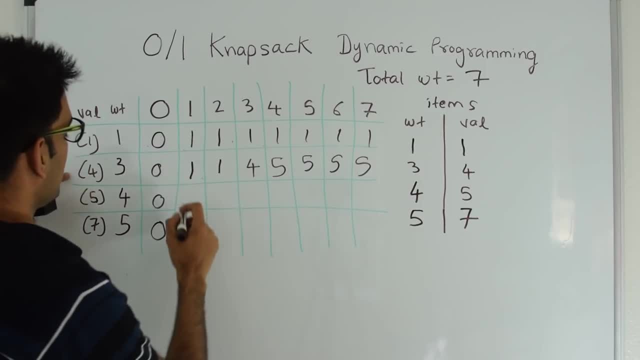 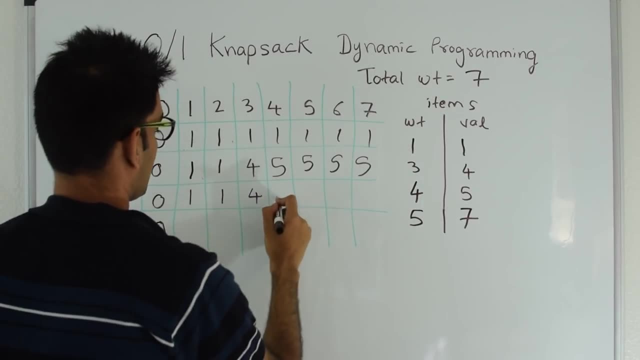 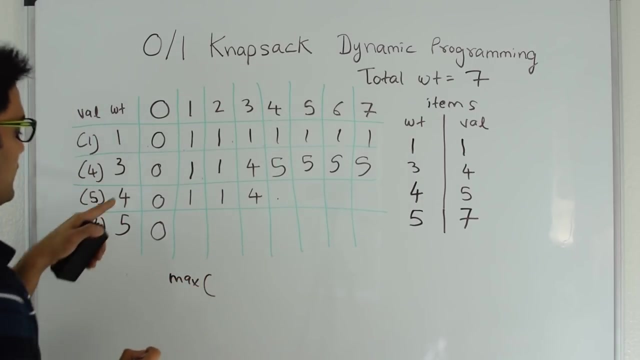 So we'll just get the value without including 4.. Without including 4, the best we can do is 1.. Similarly, 1,4.. So here at this point, if we pick 4, we'll get the max of. if we pick 4, then the best we can do is 5 plus we go up and four steps back, so that's. 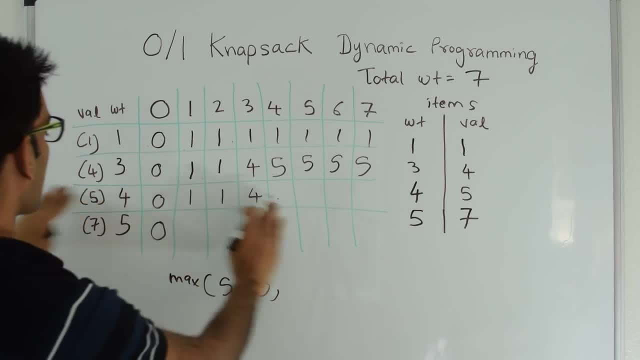 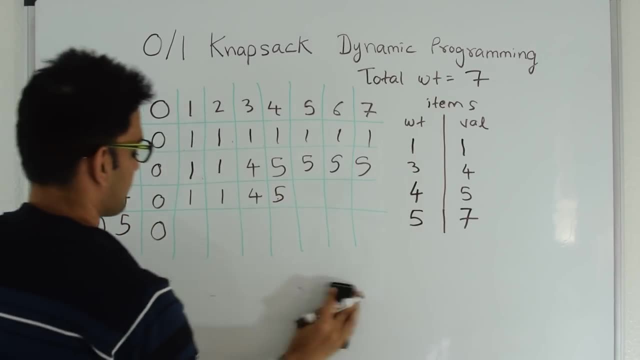 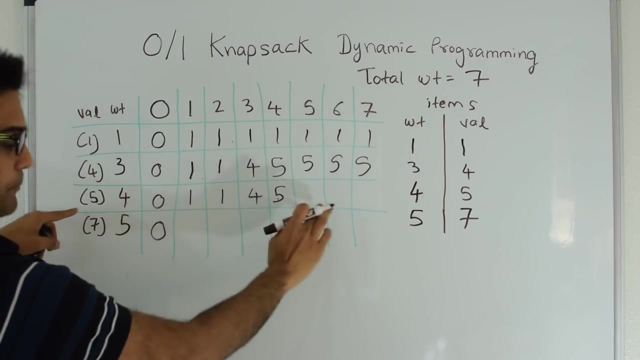 0, or the best we can do without picking 4, which is 5.. So in both the cases we get a value of 5.. So let's go here. So here, the best I can do is if I pick 4, if I pick 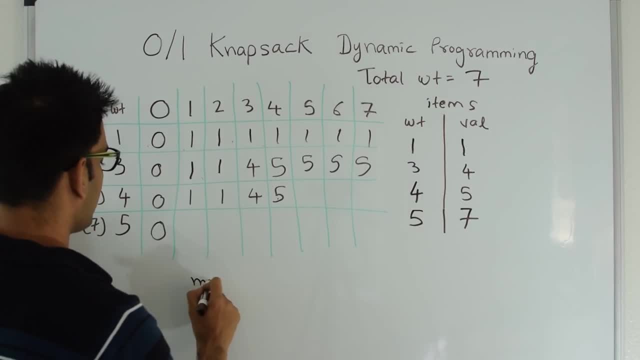 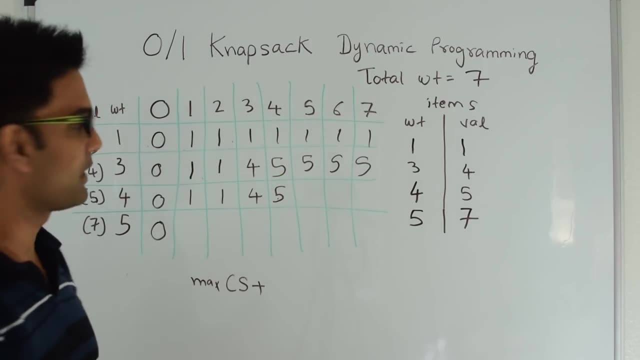 item, this item, the value this item will give me is 5 plus subtracting, subtracting 4 from 5, so we're left with one weight and we're left with two items. So if you have one weight and two items, that this value is that value. so that's. 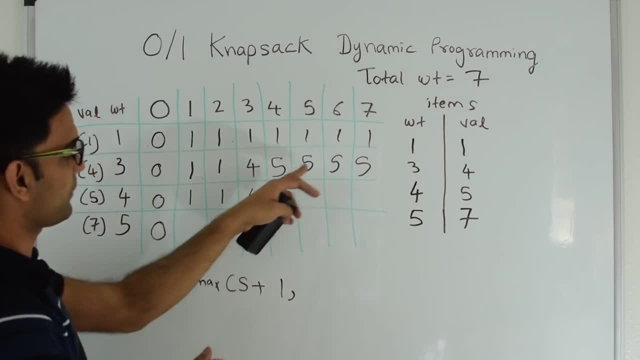 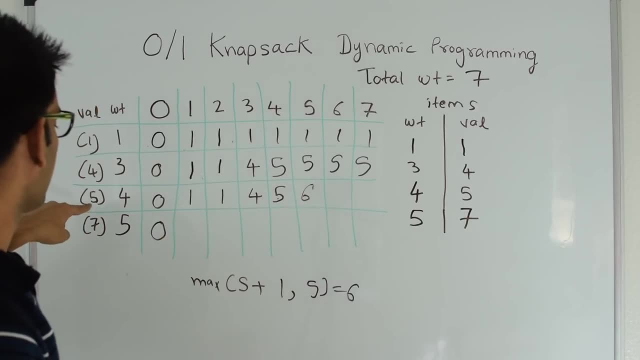 one, And then, if we did not include 4 altogether, the best I can do is 5.. So here the max is 6.. So, again, to get the 6, we get the value. we picked this item, so the value of this. 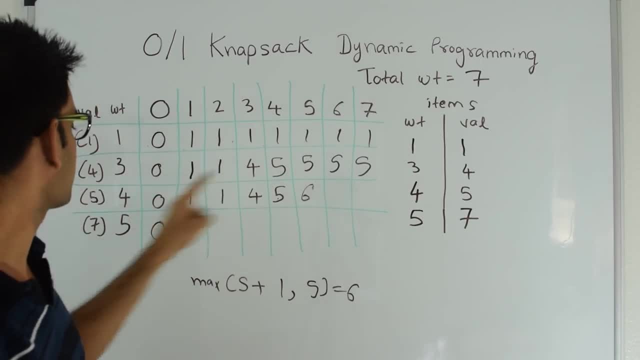 item is 5, then we go up and we go four steps back. Four steps back because 4 is the weight of this item. So 1, 2,, 3, 4 and we reach the reach this point, so we add that value to this, this value, so that value is 6. so if 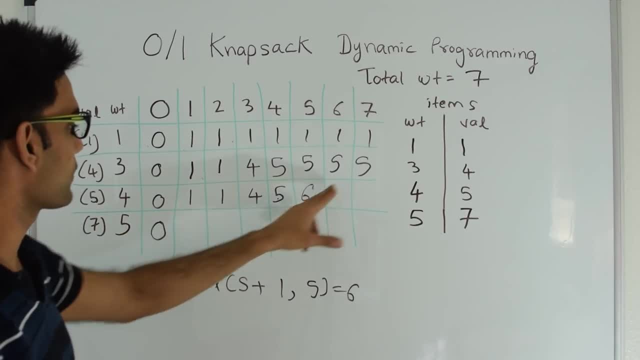 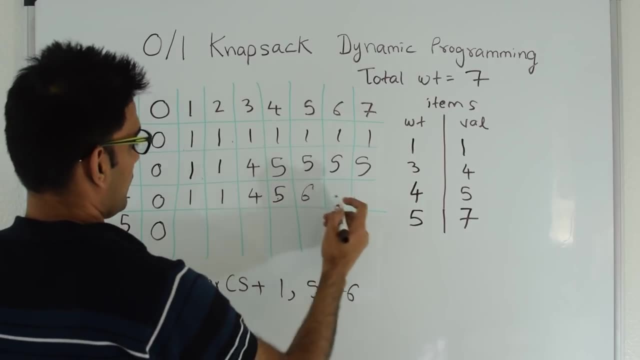 if we include 4, the best we can do is 6, and if we don't include 4, the best we can do is 5, so we take 6 here. So again for 6, the best we can do is by including this item will be 5 plus. 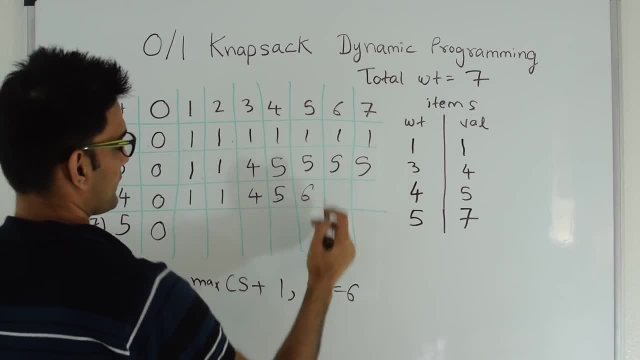 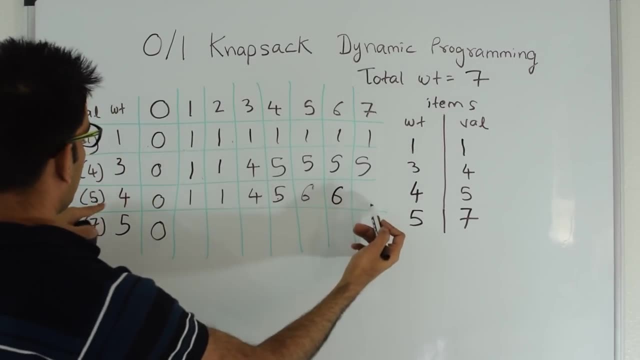 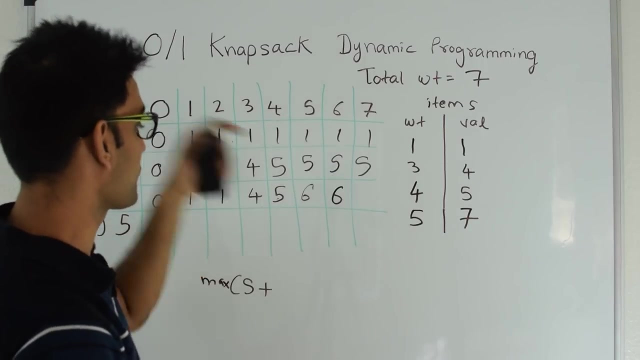 going four steps back, so that's 1,6, or this guy, so that's 6. so finally, let's look out for 7. so here, if I pick this item with weight 4, the value I'm getting is max of 4,5, plus going four steps back 1,2,3,4, so that's 4. 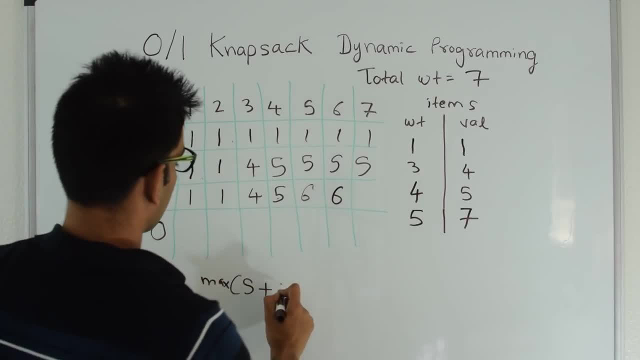 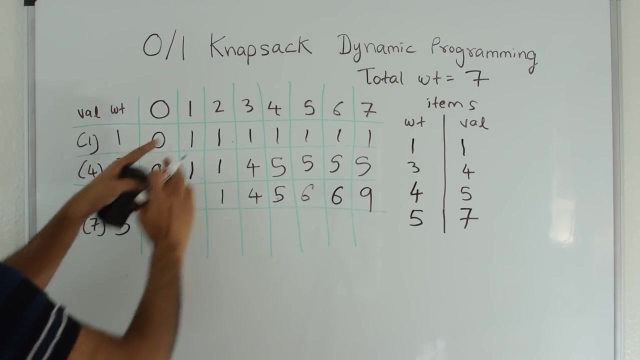 1,2,3,4, so that's 4, or not picking 4 altogether, and the best I can do with that is 5. so clearly 9 is bigger than 5, so this becomes 9.. Alright, so if we had total weight: 7 and if we had 3 items: 1,3,4- the best I can do. 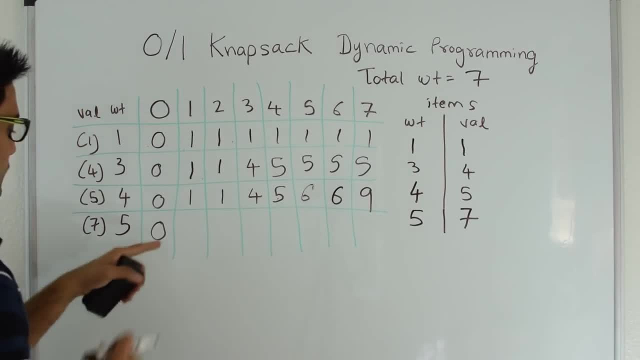 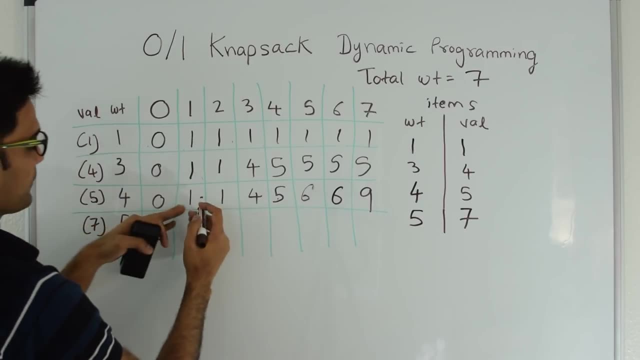 is 9. so finally, let's bring this last row into the picture. so since 5 is greater than 1, we cannot include 5 into the action, so we'll just get the value from the top, so best we can do without including 5. so that's 1, so 1,4,5, so 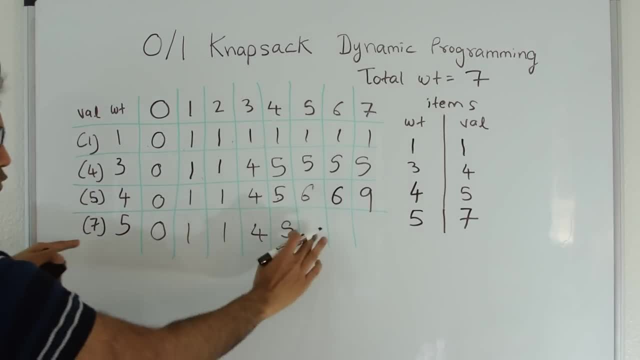 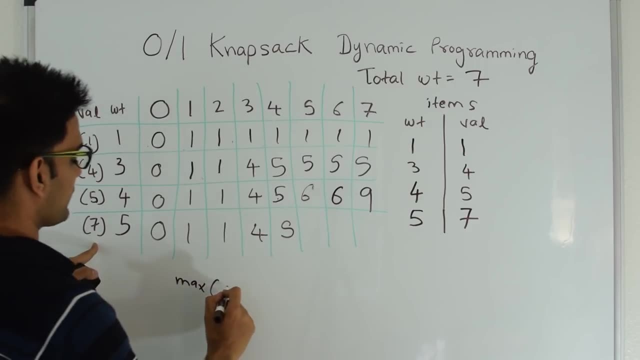 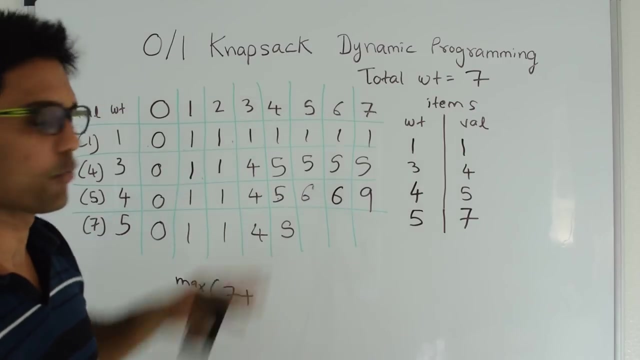 here. so the best if I include 5, if I include this 5, the best I can do is max of whatever is the value of 5. so that's 7 plus whatever is left after removing this 5 from the total weight. so we are left with 0. so 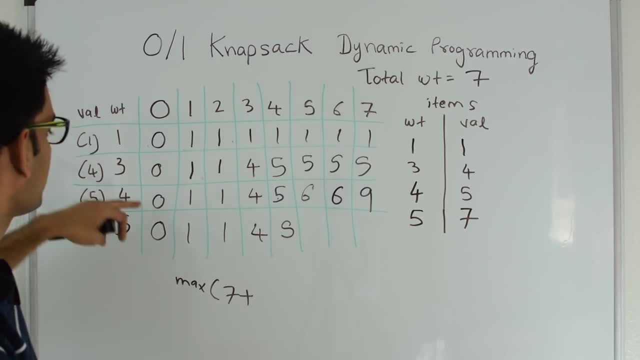 that and then with the 3 items and with the other 3 items, so we are left with 0 weight and we are left with 3 items. so that's this guy. so 0, or whatever the best we could have done without picking 5. all together, so that's 6. so here the max is 7. 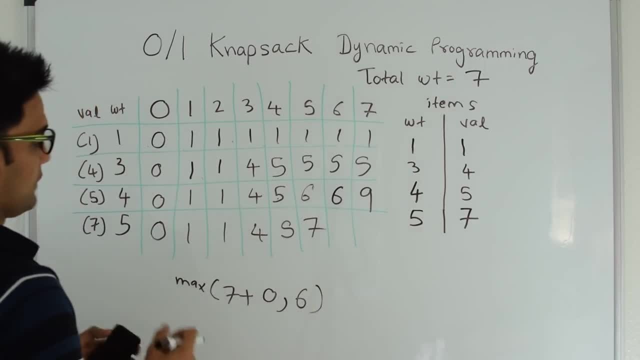 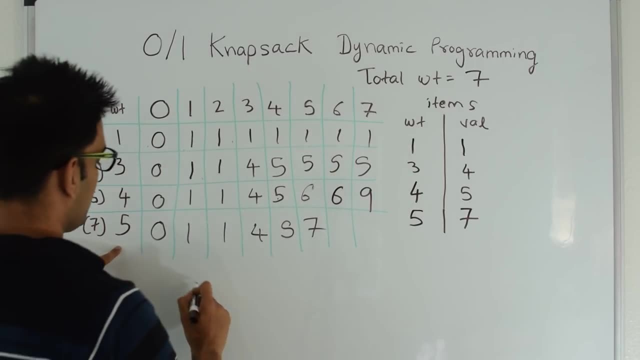 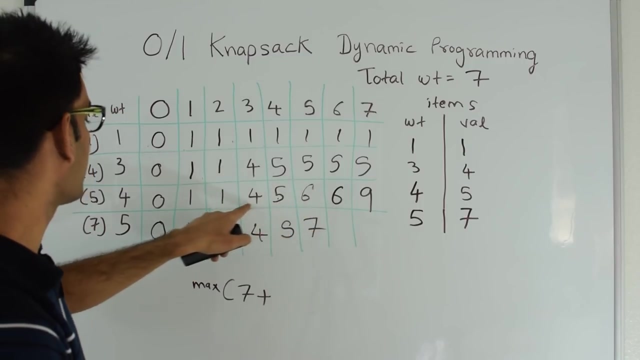 so then we come to this point. so again, what's the best we can do? if our total weight is 6, if we pick this item with weight 5, I get the value of 7, plus we go 5 steps back- 1,2,3,4,5, so 1. or if we don't pick this item all together, the 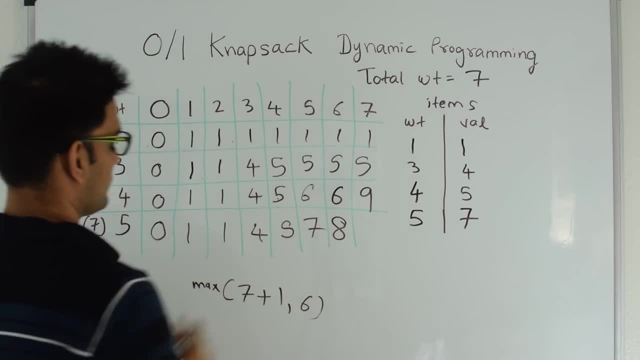 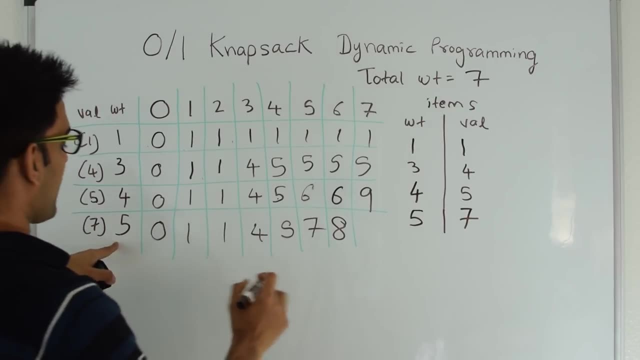 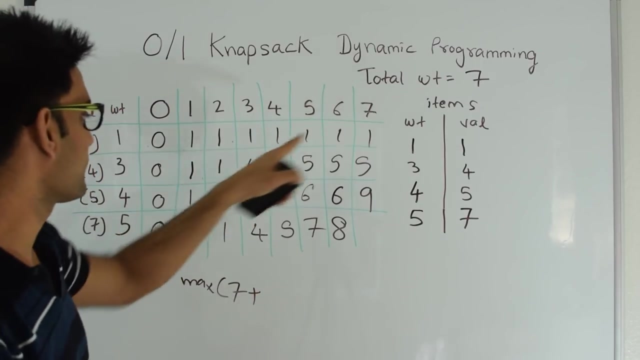 best I got is 6, so 8,8 is better than 6. finally, let's come to this point. so if I pick this item with weight 5, the value I'm getting is 7 plus I subtract 5 from 7, so I'm left with 2 and I'm left with 3 items. so basically we're. 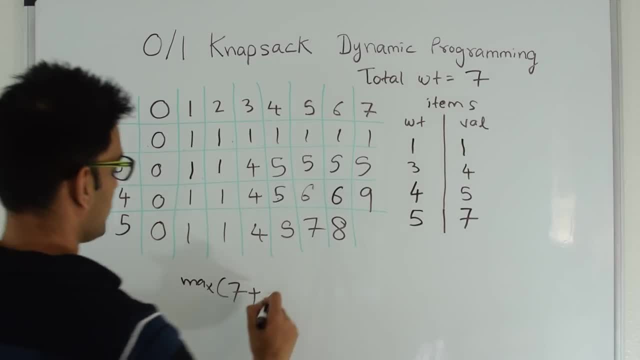 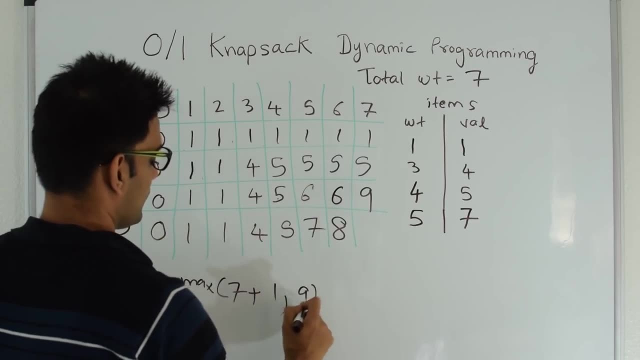 going 5 steps back here: 1,2,3,4,5 so 1. so 7 plus 1 is 8, or the best we can do without including 5. so that's 9. so here 9 is the winner. so this value is 9. 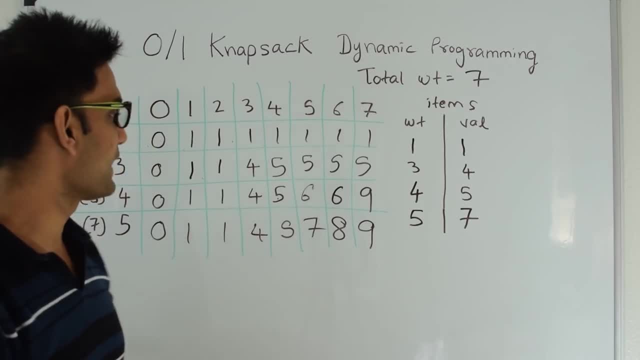 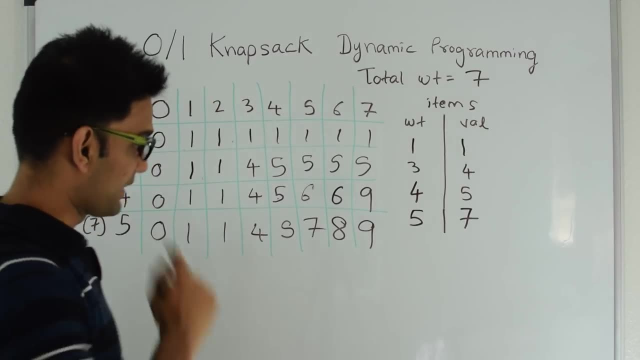 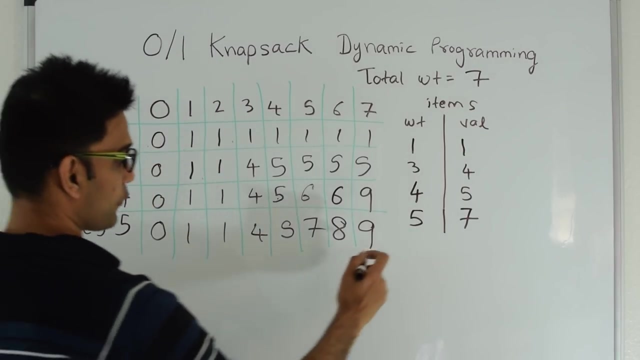 so this is the value we can, maximum value we can get- by picking items from this set such that the total weight is less than or equal to 7. so if someone asked you, what is the actual, what are the actual items which we're going to pick? so let's see how we're going to do that. so we'll start from this point here. 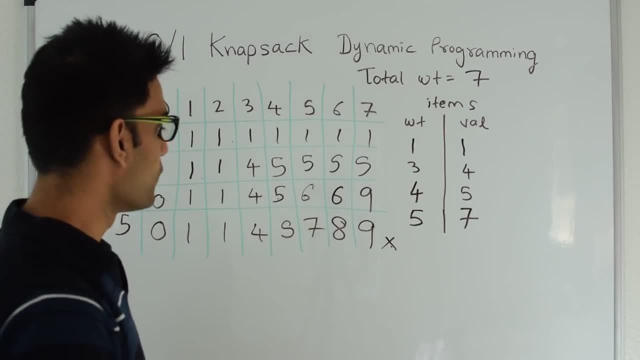 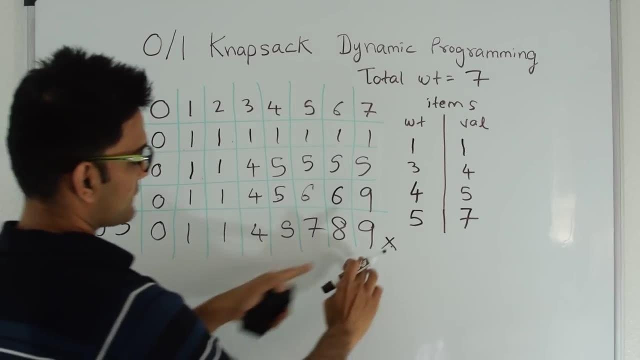 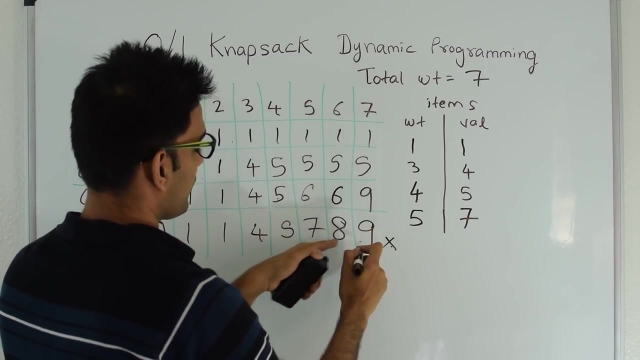 our answer and we'll move and we'll retrace back in this, in this matrix, and try to find out the actual items we are checking. where is this 9 coming from? this 9 is clearly coming from the top. it's not coming from this item. 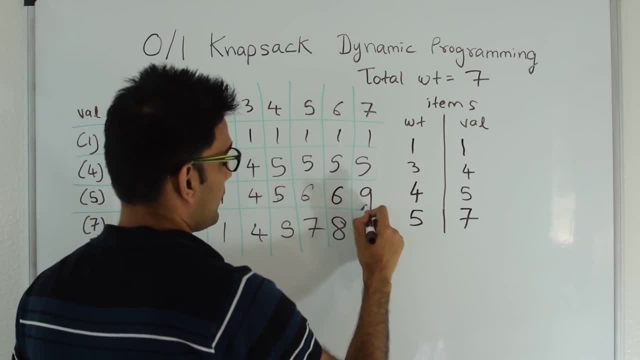 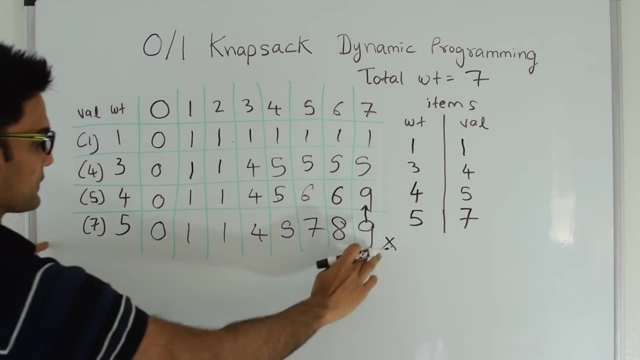 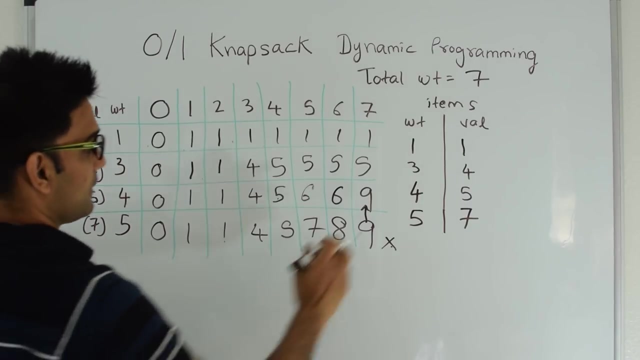 it's not coming from this item, it's coming from the top. it means that since this value is coming from the top, it means that this item is not selected. if this item was selected, this value would not be coming from the top. so we know that item with weight 5 is not in the answer. then we check: where is this? 9? 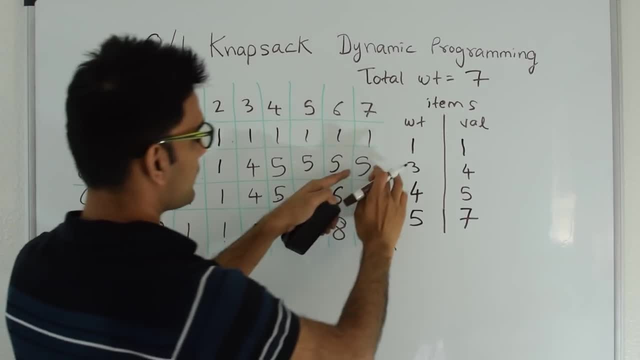 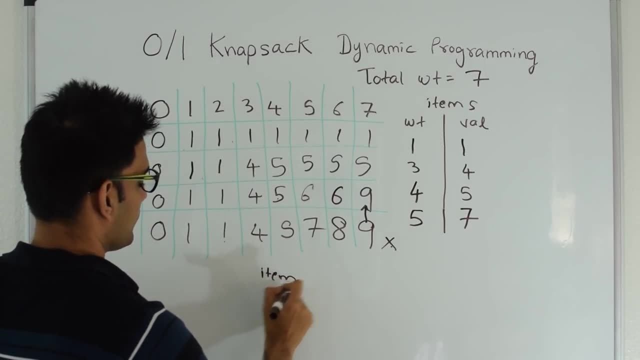 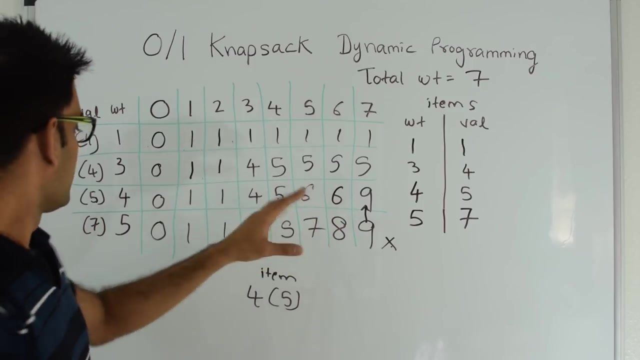 coming from this 9 is clearly not coming from the 5, so this item must be in the answer. so item 4 with value 5 must be the answer then. so this item is selected, then we say: where do we go from here? so then we go up and we go four steps back: 1, 2, 3, 4, so 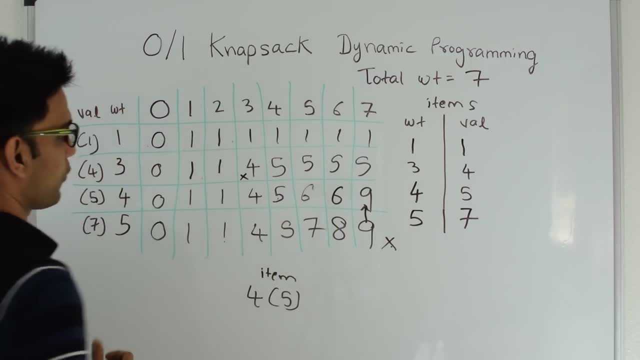 this point. so from here we directly go to this point. since this item is selected, it means that it must be taking 4 weight. so whatever weight we are left with, which is 3, and whatever two items we are left with, that is where we're going to end up next. so 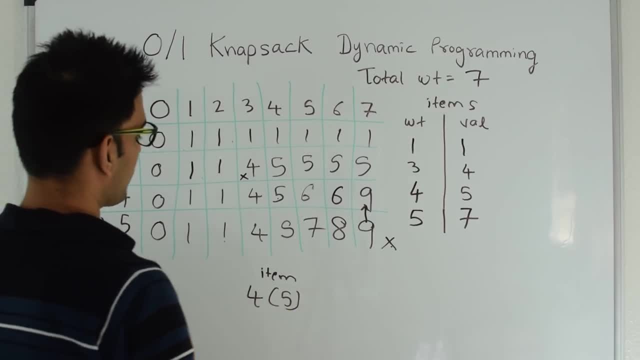 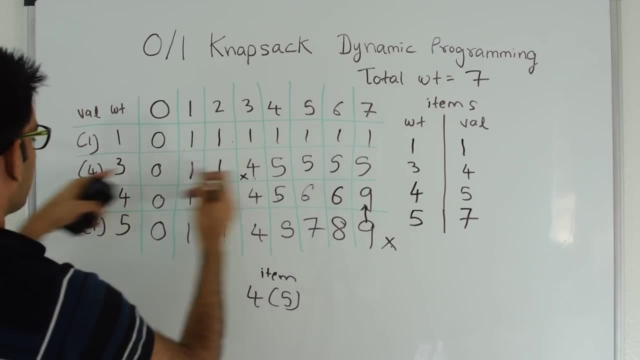 that's this point. so item with weight 4 and value 5 is selected, then we check: where is this guy coming from? this guy is not coming from the top, so this guy, this particular row, also must be selected. so the item with weight 3 and 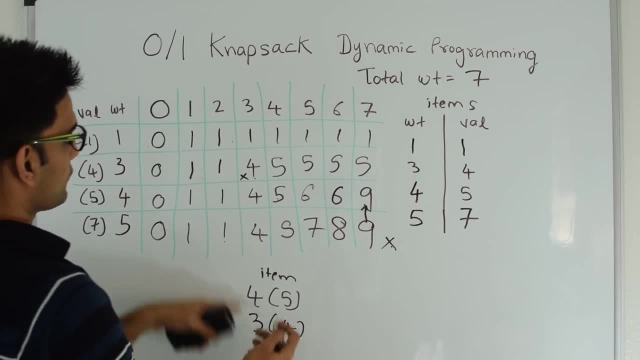 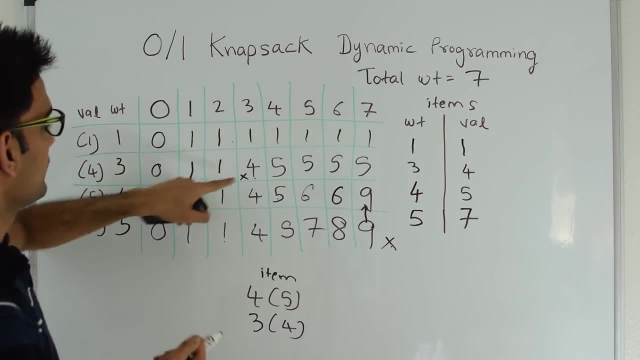 value 4 is also selected. so again, now that this item is selected and the weight of this, the weight of this item is 3, so we go up and go three steps back and reach this point. as soon as we reach a point where the weight is, 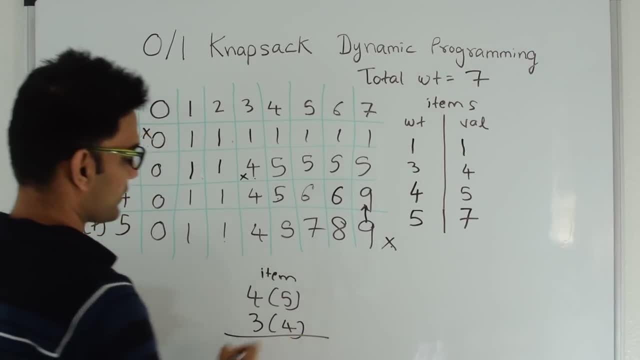 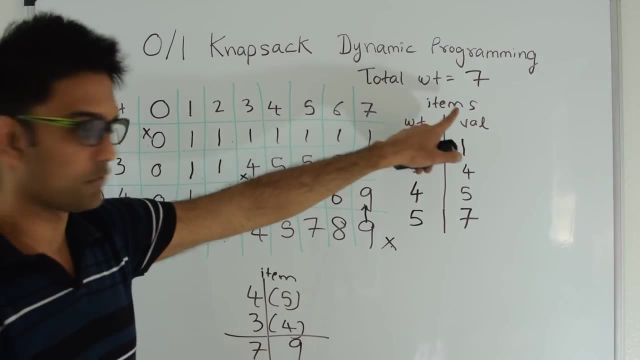 0. we are done. so, basically, these two items are our selected item and the total value here is 9 and total weight is 7, so total weight is less than equal to the sum of the weight is less than equal to total weight and the value is maximum. 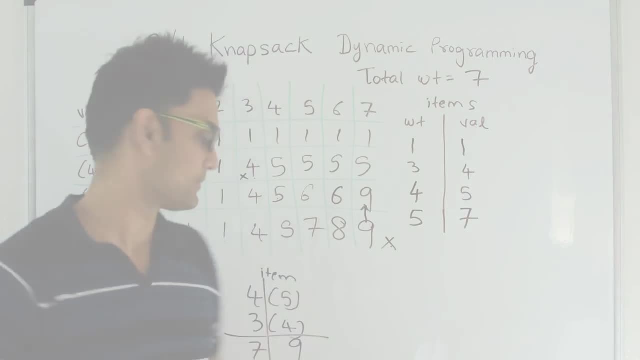 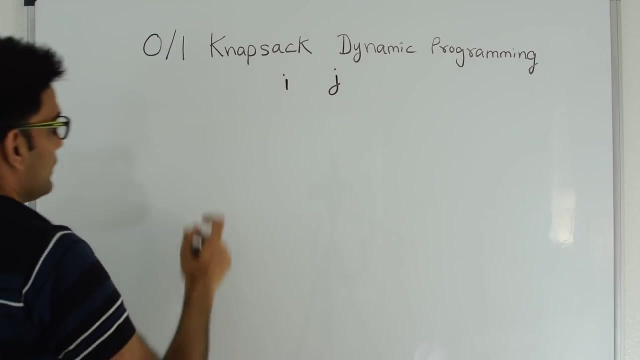 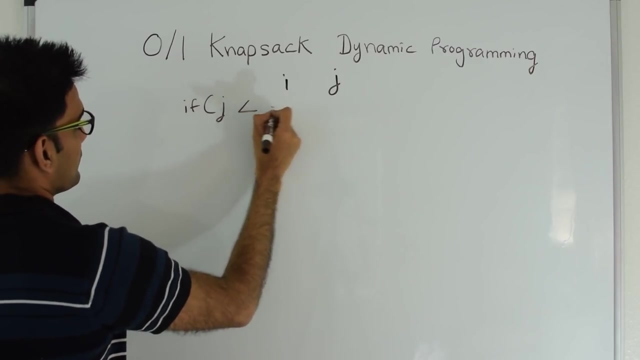 next let's look at the formula for this problem. so here, I is my column and J is my. I is my row and J is my column. so if J, which is my weight, is less than weight of I, so weight of item I, it means that I cannot.